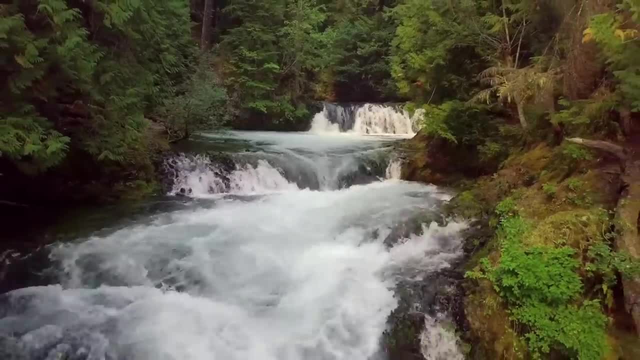 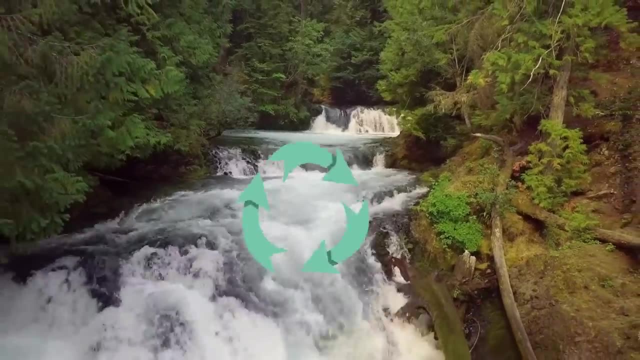 Air and water are renewable natural resources also. They don't regrow like trees, but they are always being renewed. A renewable resource is a natural resource that is used by humans. A natural resource can be replaced within a person's lifespan. They move in cycles, Remember: renewable resources can regrow or be replaced within a person's. 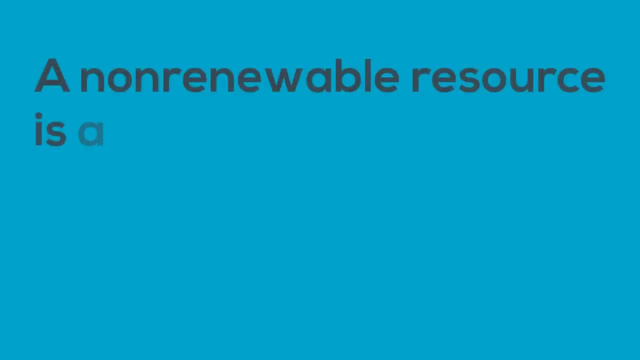 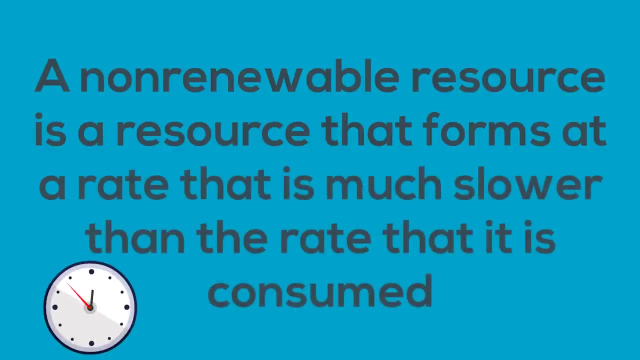 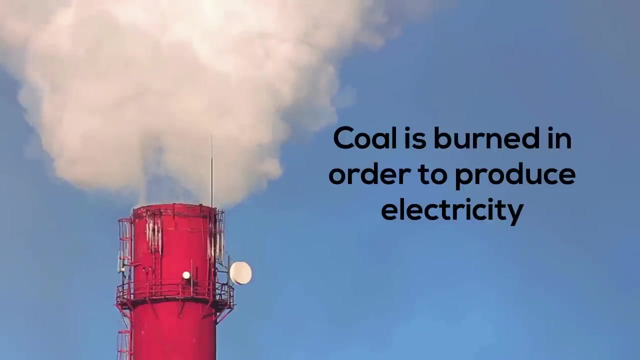 lifespan. A non-renewable resource is a resource that forms at a rate that is much slower than the rate that it is formed. Coal is an example. It takes millions of years to create coal and once it is used up, it is no longer available. You can use the phrase con to remember three. 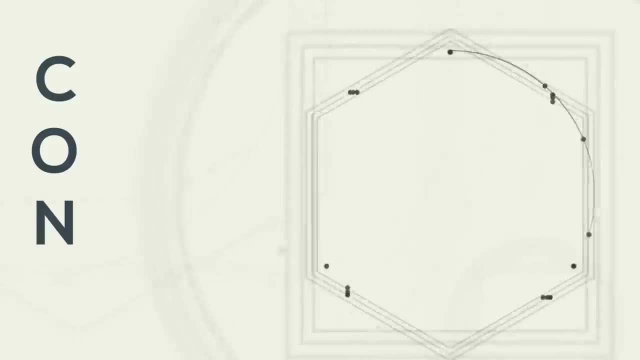 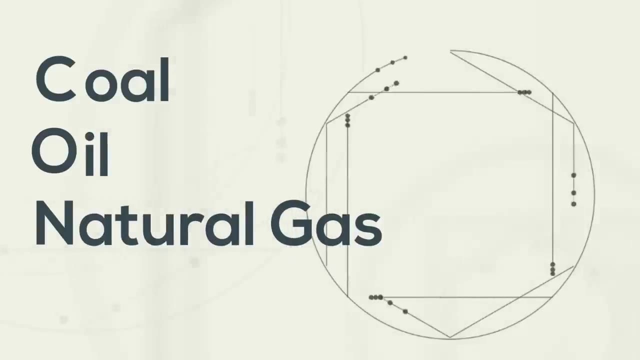 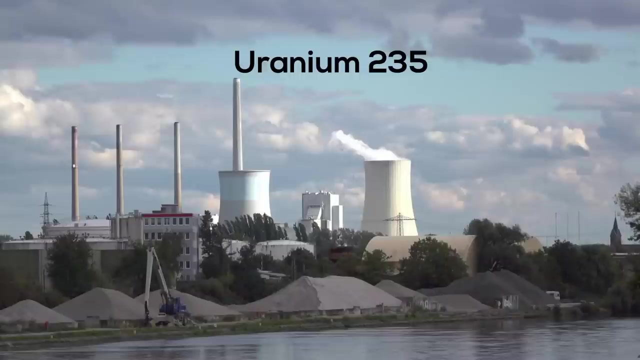 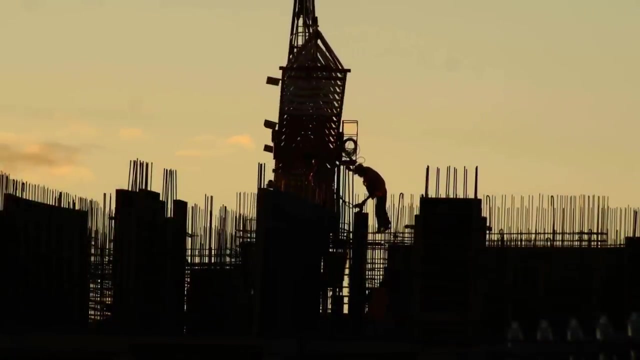 popular non-renewable resources. This stands for coal oil, natural gas. Nuclear fuel is also a non-renewable resource. Uranium-235,, which is used in nuclear power plants, is found in a finite amount. Minerals used for making metals are also non-renewable. 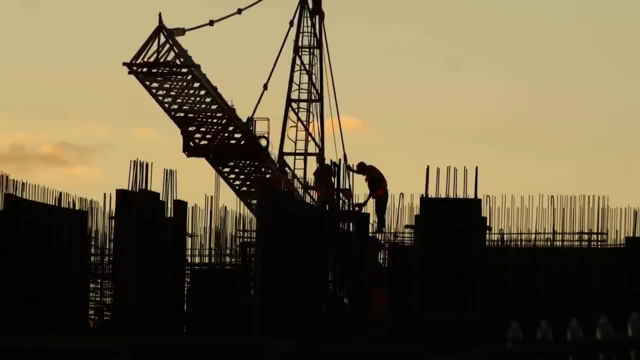 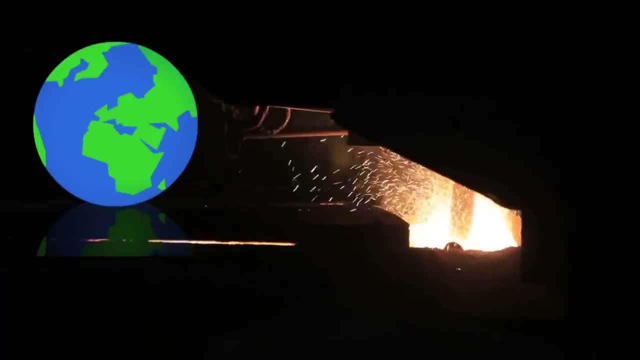 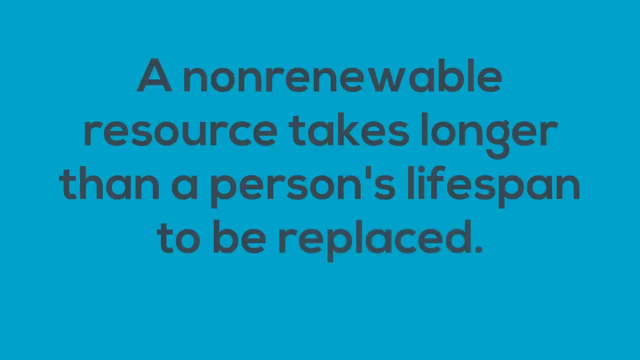 For example, steel, which is used in making buildings, is made of iron ore. Iron ore is mined from the earth and is a limited resource. Non-renewable natural resources are things that take longer than a person's lifespan to be replaced. In fact, it takes millions of. 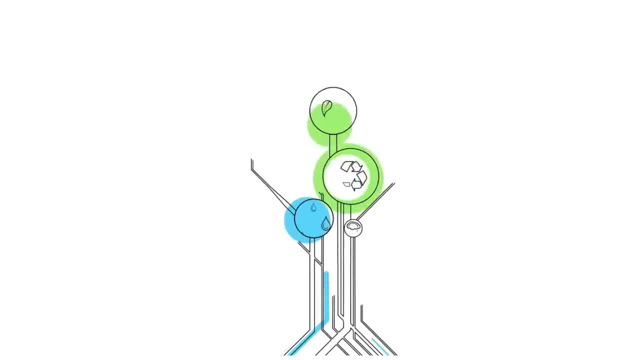 years to form these, Because many important resources are limited. we can all reduce, reuse and recycle. You can turn off lights when you're not in a room. You can ride your bike more and walk more to improve your life. You can use a natural resource to help you improve your life. 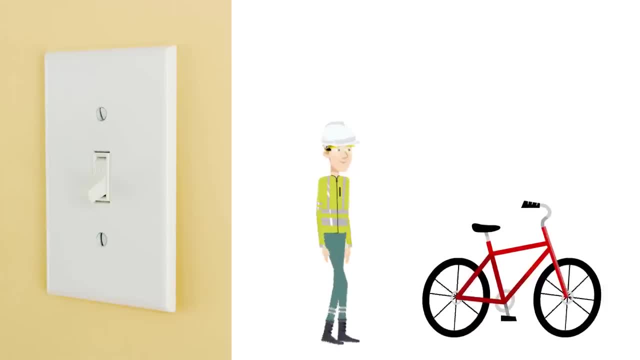 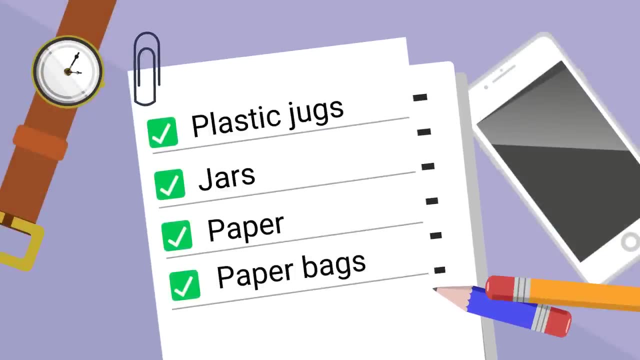 You can reduce the amount of gasoline used. You can reuse and recycle things like plastic jugs, jars, paper, paper bags, plastics, cardboard, aluminum and even steel. If you'd like to know more about how we get energy from non-renewable resources, this playlist will. 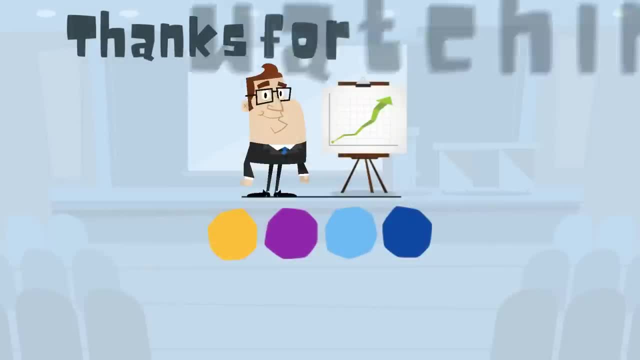 help. Thanks for watching, and MooMooMath uploads a new math and science video every day. Please subscribe and share. See you next time.